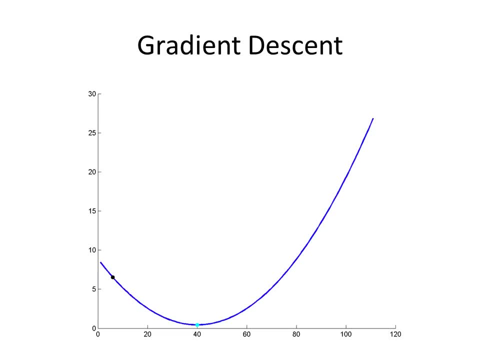 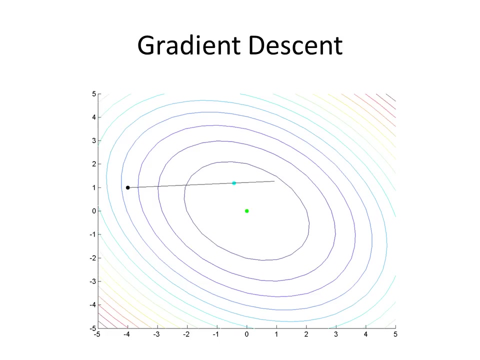 gradient line. This is relatively easy and we can employ many different methods to do this, including Newton's method. Once we have found the minimum along the gradient line, we can look at it on the isocontour graph. Notice that the minimum along the gradient line is closer to the goal. 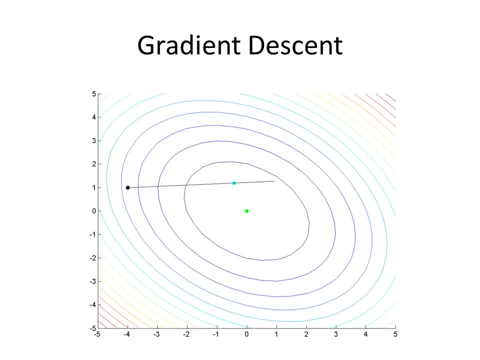 than the original point. We can use this minimum along the gradient line as the next guess of the minimum point. We can then compute the gradient at this new point. Notice that this new gradient must be orthogonal to the previously computed gradient. If it was not orthogonal, that means that 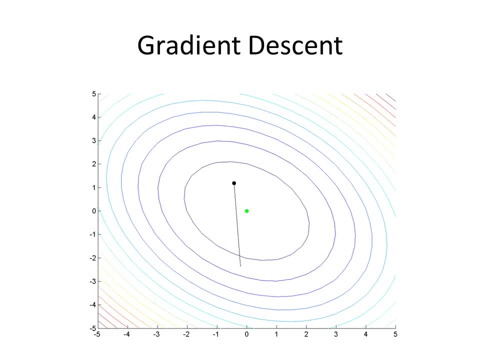 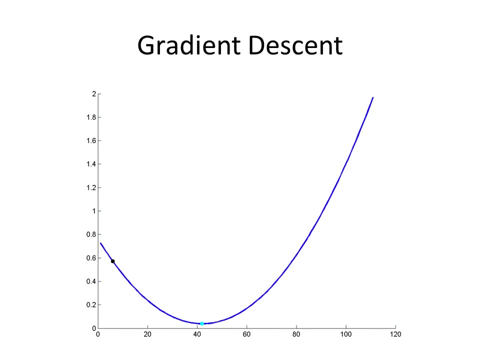 there is a component that is along the previous gradient. This means that we could travel further along the previous gradient to reach a more optimal point, We again find the minimum of the section of the curve that is along the gradient line. Once we have found the 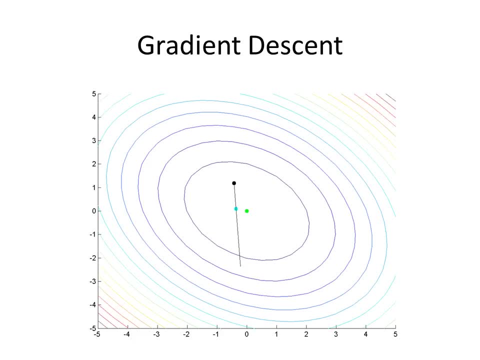 minimum. again, this will be closer to the goal than the original point. We can now use that as our next guess. Our final path, once we have done this several times, will look somewhat like this: One problem with gradient descent is that this path will form a zig-zag and this path will form a. 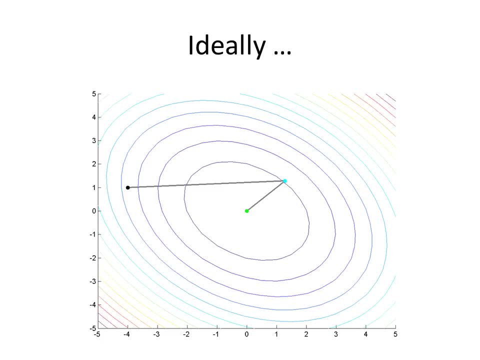 straight line. Ideally, we would have liked to take a slightly larger step than we did and reach a point for which the next step led directly to the goal. Even better would be to take a step along the gradient, such that the gradient at the next point would 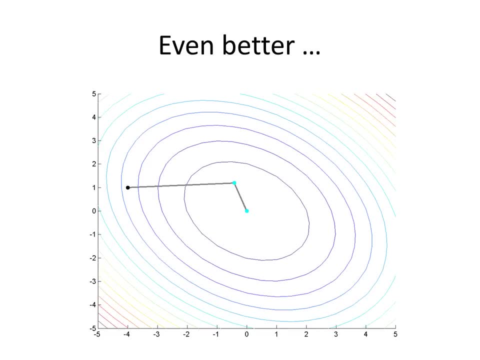 still be orthogonal and would reach us to the goal. This is the key idea behind the conjugate gradient method. Suppose we had an n-digit, n-dimensional feature space. In the conjugate gradient method we search n conjugate directions such that progress made in one direction does not affect progress made in the other directions. 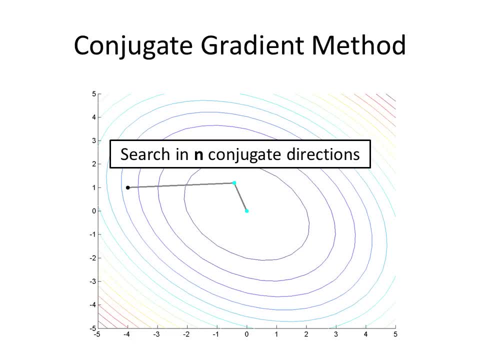 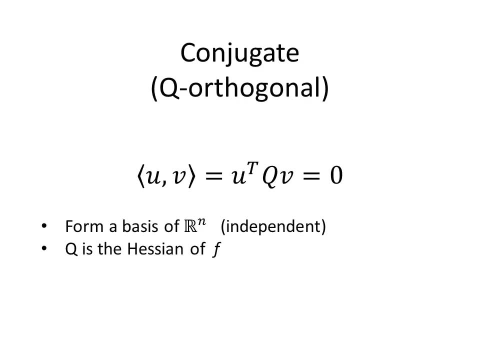 Thus we only need to search in n directions to find the optimal point For two vectors to be conjugate or Q-orthogonal. we can define the inner product of the vector as a new vector. The vector's inner product is a new vector and the vector's inner product. 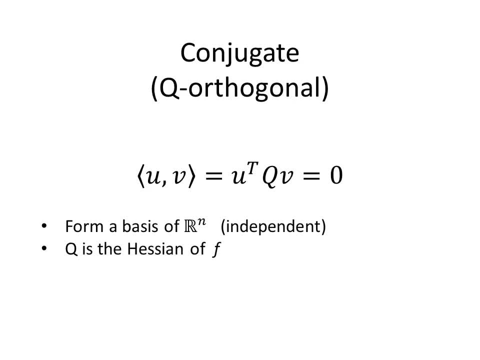 of the two vectors u and v. as u transpose qv. If the two vectors u and v are conjugate, then the inner product will be zero. A set of n, q orthogonal vectors will form a basis of our n. This means that they are all independent. In our case, q is the hessian of f, the function. 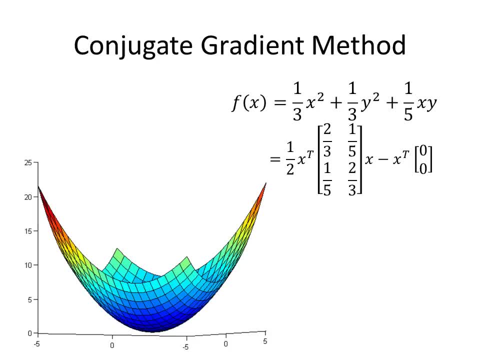 we are trying to minimize Specifically for our initial minimization problem of f of x equals 1 third x squared plus 1 third y squared plus 1 fifth xy. we can rewrite this function as 1 half x transposed. This generalized version of the function will be used to demonstrate the conjugate. 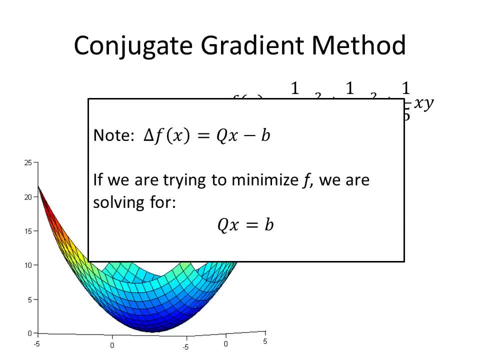 gradient method. Note that the gradient of this generalized function is q. If we are trying to minimize f, we are solving for when this gradient is zero, specifically when q is equal to b, In order to use the conjugate gradient method. suppose we had. 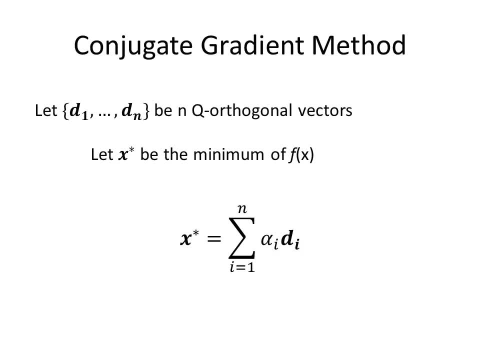 n, q. orthogonal vectors d1 through dn. We can represent the minimum of the function f of x. let us call this variable x star as a linear combination of these n orthogonal vectors. As we said before, the vectors d1 through dn span are n. Thus we can represent: 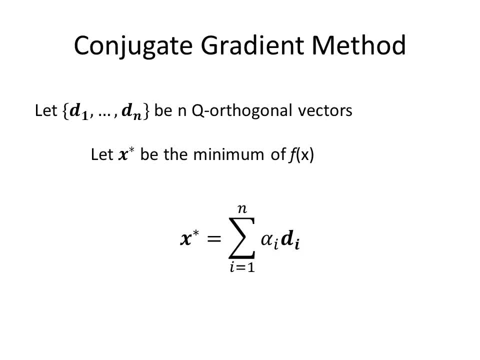 any vector as a linear combination of the q orthogonal vectors. Looking at this equation again, we can multiply both sides by the matrix q. Notice that q is equal to b at the minimum. Thus we have that b is a linear combination of q times the original q orthogonal vectors. 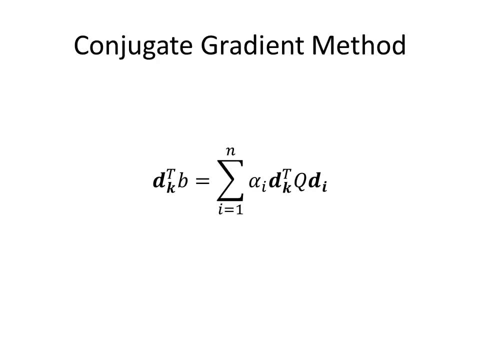 If we multiply both sides by one of these vectors, say dk, we notice that the vectors dk and di are q orthogonal. This means that for every value of k not equal to i, the inner product is zero. Thus we can simplify this equation as follows. This simplified equation: 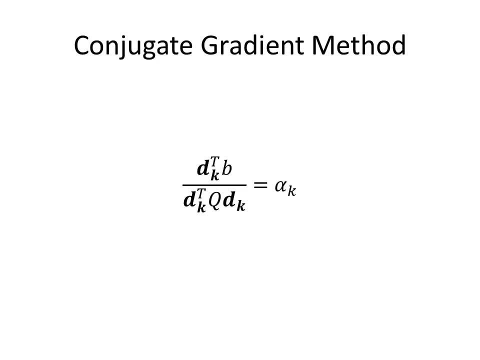 allows us to solve for alpha. 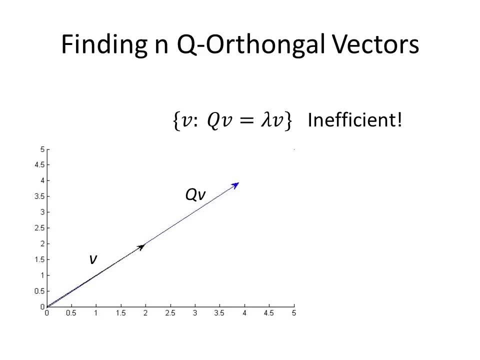 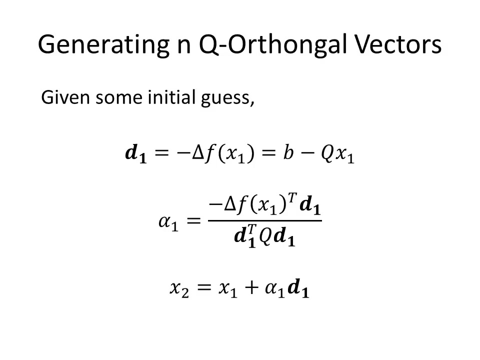 We can do this by finding the set of vectors V, such that Q times V is equal to some constant lambda times V. This set V are the eigenvectors of the matrix Q. In general, finding the eigenvectors is inefficient. A better method to find n-Q orthogonal vectors is to generate them dynamically, Given some initial. 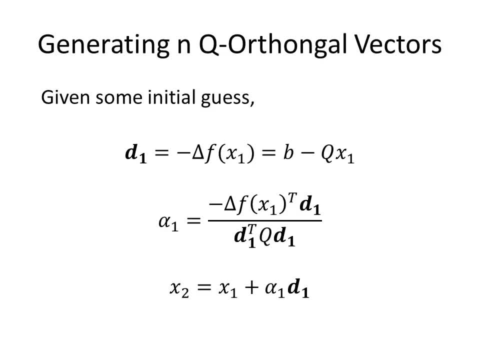 guess x1,, we can calculate the first orthogonal vector as the negative gradient. We can then calculate the corresponding alpha with which we can increment the initial guess to get the second guess. In order to calculate the second orthogonal vector, we must first calculate the gradient. 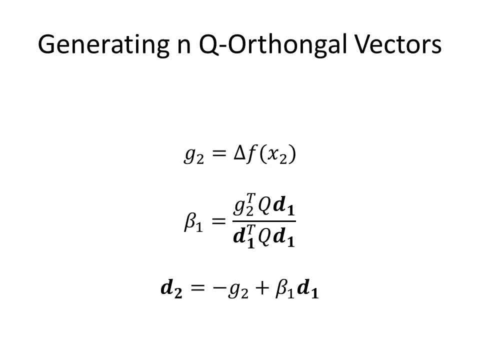 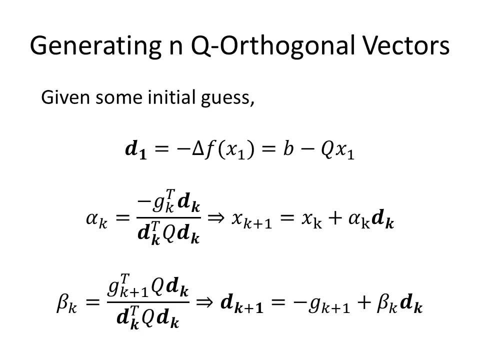 at this new guess, g2.. We can then use that to calculate a step size along which we can increment g2 in order to get the new orthogonal vector. In general, we can generate n-Q orthogonal vectors and find the minimal solution as follows. 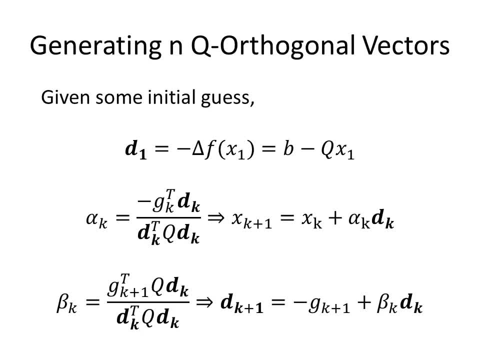 Given some initial guess- x1,, we can calculate the first orthogonal vector as the negative gradient evaluated at this initial guess. We can then calculate the value for alpha and use that to update our guess. We can then calculate beta and use that to update the value of the orthogonal vector. 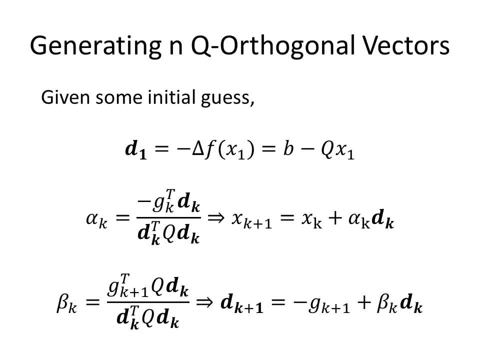 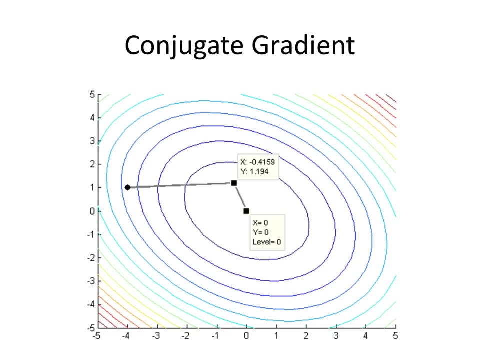 If we do this iteratively, we end up with a final value of x that is close to our optimal solution. We now see the conjugate gradient method in action on our original problem. In the first iteration the algorithm takes a step size of 1.4 along the 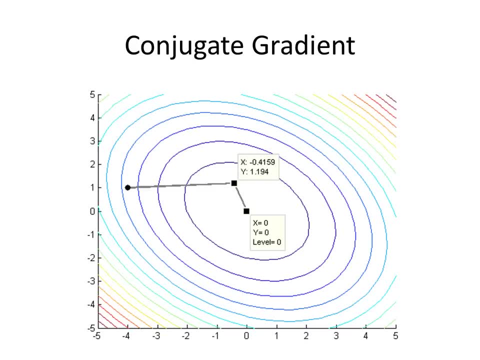 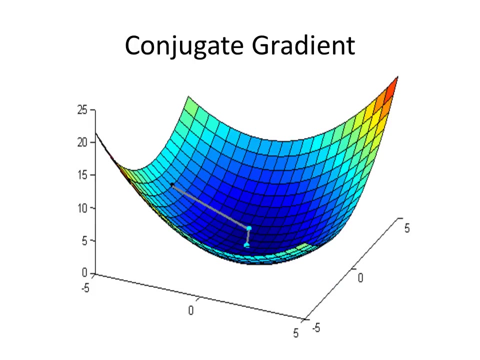 gradient to reach the point negative 0.41, 1.19.. In the second iteration the algorithm takes a step size of 1.7 along the gradient to reach the optimal solution within 10 to the negative 16th. This concludes the video lecture on conjugate gradient method. 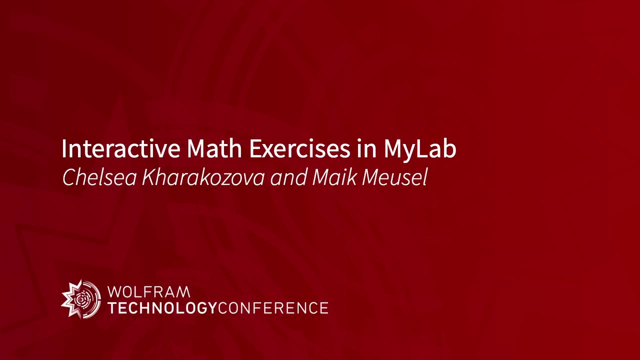 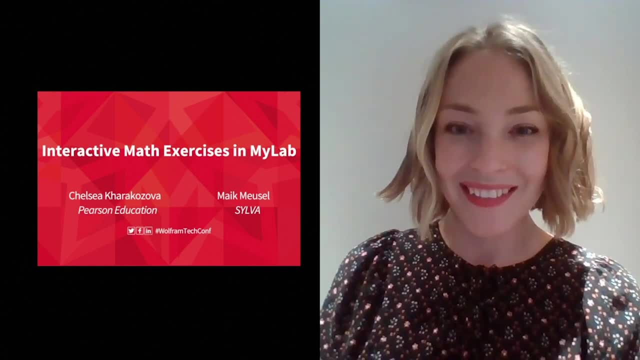 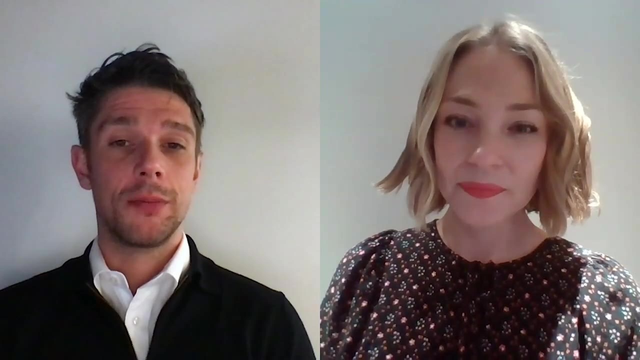 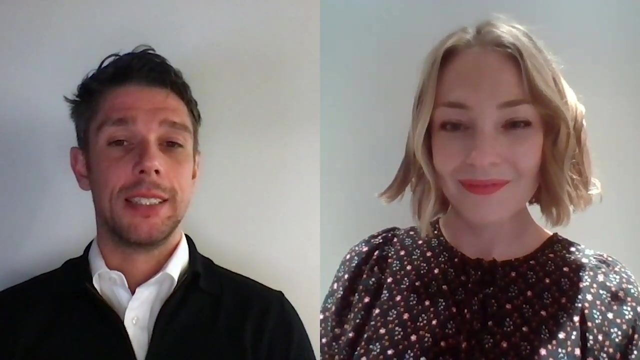 Hi, I'm Chelsea Karakozova. I'm a product manager for STEM math products at Pearson and I'm based in Boston. Hi, I'm Mike from SILVA, a Zurich-based edtech startup using Wolfram technologies. In our presentation, we show how SILVA helps Pearson to create interactive math exercises. 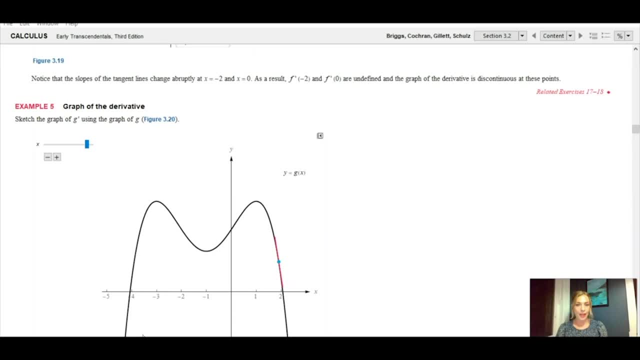 I work at Pearson as a product manager on our MyLabMath platform, which currently serves millions of students in the US and worldwide. MyLabMath is a fully-featured content and assessment platform. Students come here to read the e-text, do practice homework and even take high-stakes. 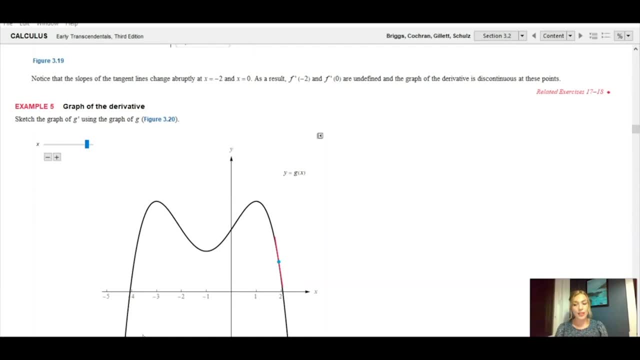 assessment. Where we do see a bit of a gap is in our assessment questions. We have a bank for each title of thousands of questions that consist of multiple choice, free response, drag and drop, interactive video, But we have a consistent request from faculty to drive conceptual understanding and to really